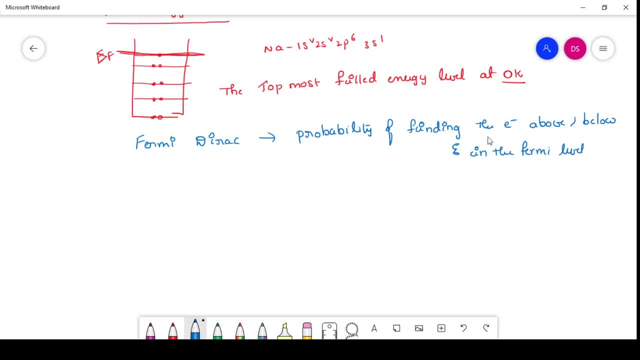 That means how the conduction process takes place as per the quantum concept. So if you can give a little bit of energy, Okay. so If the energy electron absorbs and it jumps into the empty levels, then those electrons participate in the conduction process. 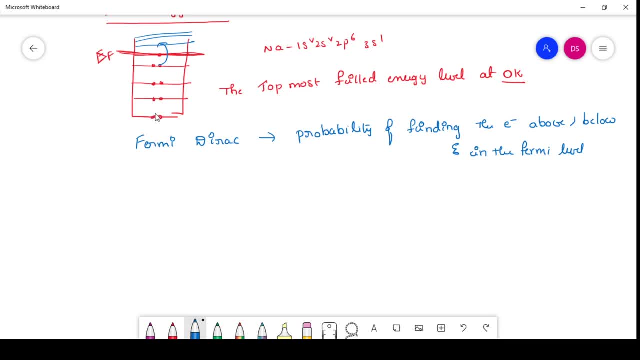 And there will be no excitation takes place in between the filled energy levels, As per the quantum concept. they have explained like this: Now, Fermi Dirac distribution explains how the occupation of electrons will be above the Fermi level, below the Fermi level and in the Fermi. 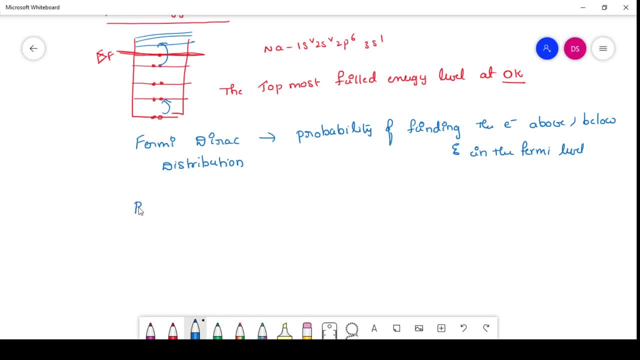 So the Fermi and Dirac have given one equation is probability of finding the electron. P of E is equal to 1 by E power, E minus EF by KT plus 1.. E is the energy of the electron in a particular energy level, EF is the energy of the Fermi level and K is the Boltzmann constant. 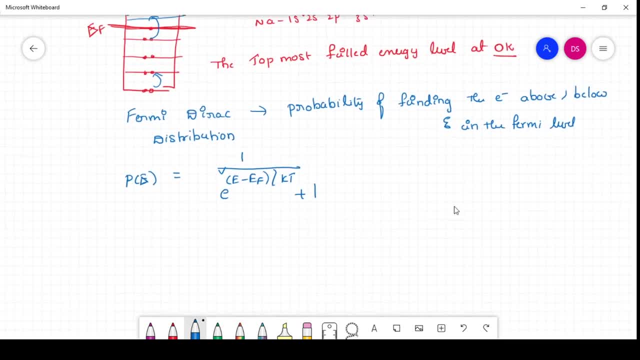 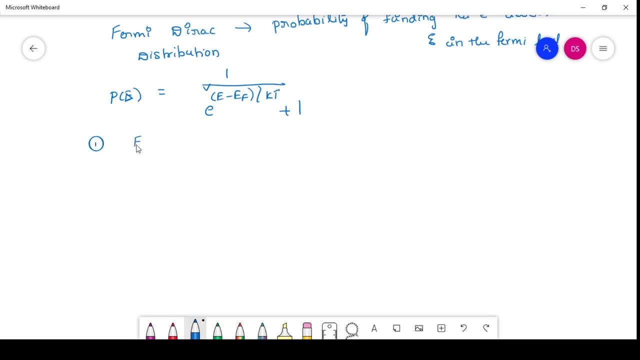 T is the temperature. Okay, so, According to the Fermi Dirac distribution. So they have considered the three cases- In the first case they have taken, the energy of the electron is less than energy of the Fermi level at T is equal to 0 Kelvin. 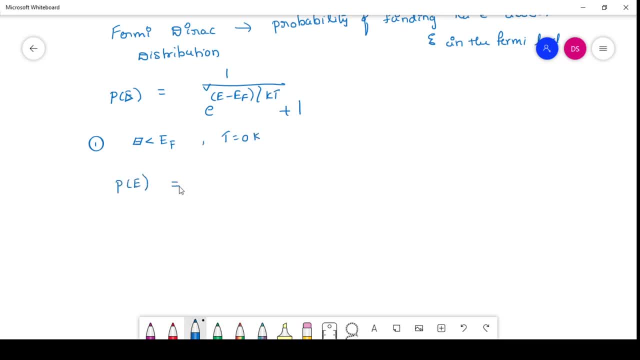 Then what will be the probability of finding? the electron P of E is equal to 1 by 1 plus E power, E minus, In this case E minus EF is E is less than EF and E minus EF becomes a negative. So negative value by temperature is 0.. 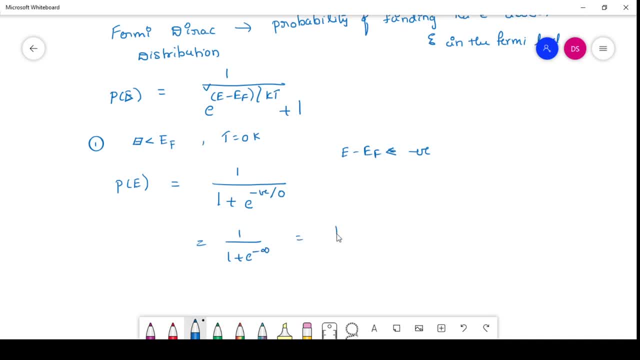 So 1 by 1 plus E power minus infinity and 1 by 1 plus, we can write E power infinity. So 1 by 1 plus 1 by E power infinity is nothing but 1 by infinity, It is nothing but 0.. 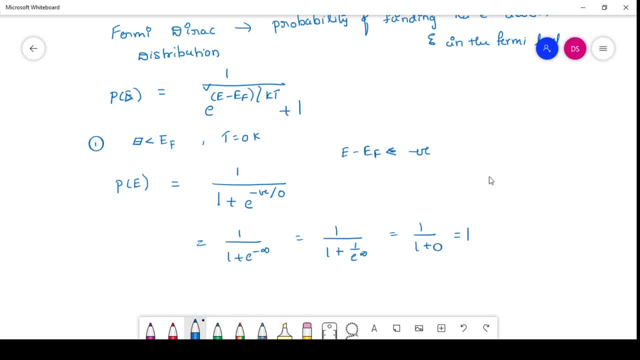 That is a 1.. So when energy is less than Fermi energy of the electron is less than Fermi energy level, That means there is a probability of finding the electron is 1.. That means the levels which are below the Fermi energy level you can find the electrons. 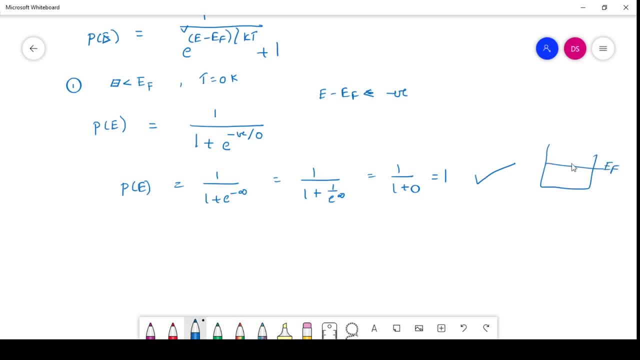 You can see the diagram. So the top most filled energy level is nothing but the Fermi energy level, And below the Fermi energy level all the energy levels are filled. Filled states are Available Now. in the second case, if you can see, E is greater than EF and T is equal to 0 Kelvin. 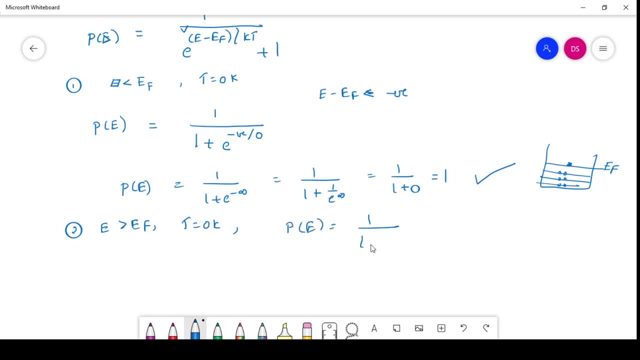 Then the probability of finding the electron becomes 1 by 1 plus E power positive by 0. That means 1 by 1 plus E power infinity. The value becomes 1 by infinity, That is equal to 0. That means when the energy is greater than EF. 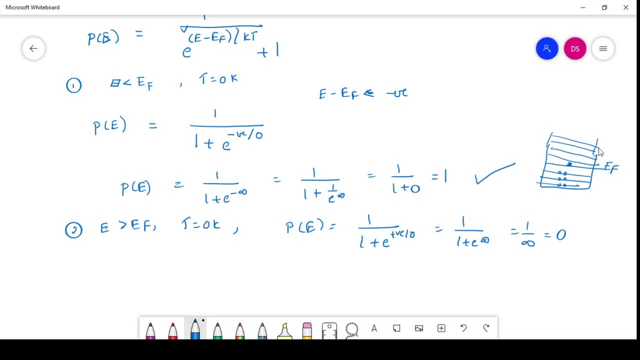 That means the states which are having the energy values greater than EF. the probability of finding the electron is 0. That means the energy levels which are above the Fermi level all are empty And the energy levels which are below the Fermi level all are filled states. 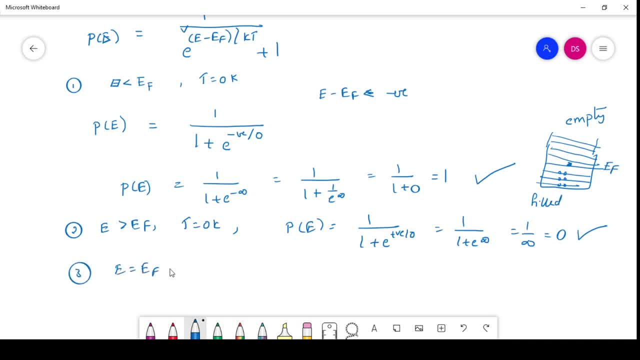 Now, in the third case we will see, E is equal to EF, And here, in this case, T is not equal to 0 Kelvin, It is greater than 0 Kelvin. The probability of finding the electron P of E is equal to. 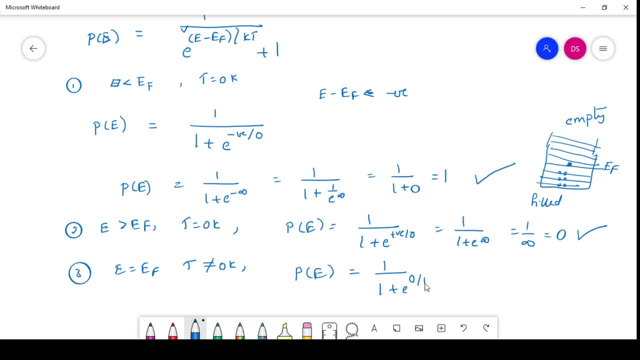 1 by 1 plus E power: 0 by KT, Because it is not 0 temperature. 1 plus E power: 0.. 1 by 1 plus 1. We will get 1 by. That means 50% of electrons are available in the Fermi energy level. 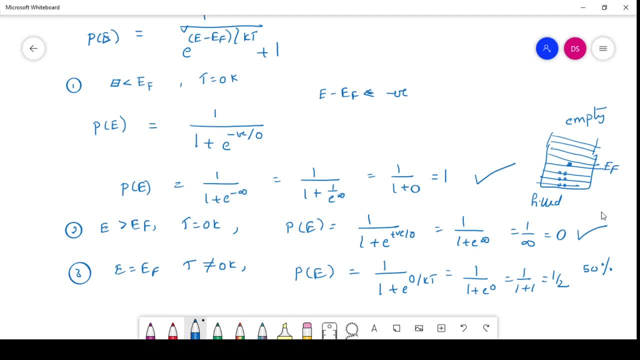 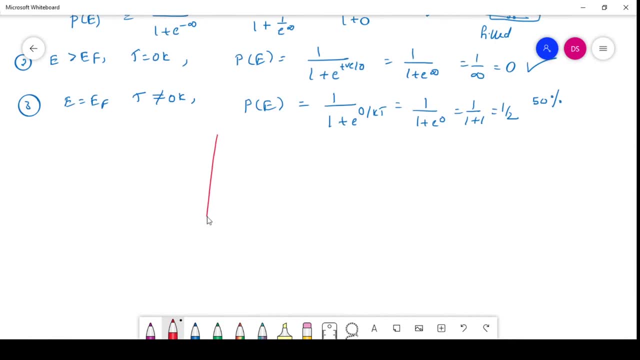 So there is a 50% of chance of finding the electron. So what are the final conclusions of the Fermi direct distribution? So they have explained as simply in one graph: On x-axis they have taken the energy And on y-axis they have taken the probability of finding the electron. 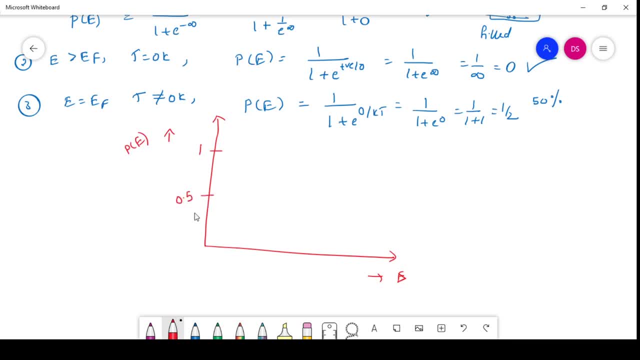 So two cases. One, they have taken the value 0.5 and 0.. So Okay, So below the Fermi- this is the at the Fermi energy level- what is the probability of finding the electron 0.5.? 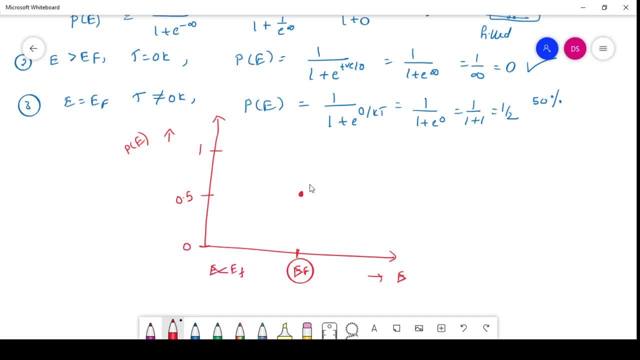 And when the energy value is Less than EF, The probability of finding the electron is more. That means this graph tends towards 1.. Okay, Then, if energy is greater than EF, This graph tends towards 0.. Because the probability of finding the electron is 0..